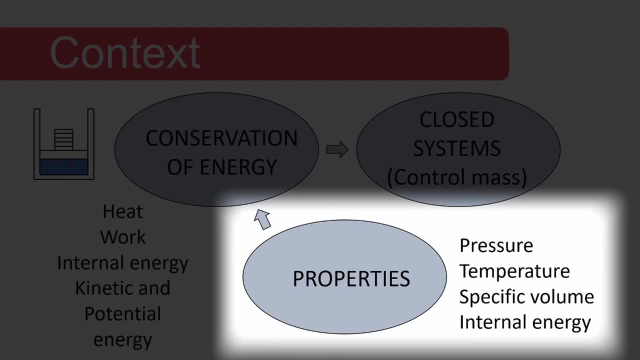 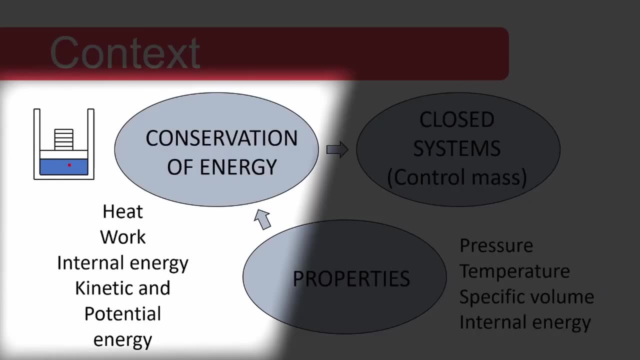 of substances, and initially we only discussed pressure, temperature and specific volume, But later saw that internal energy is also a property. Then we encountered the concept of conservation of energy, which states that energy cannot be created or destroyed. This concept is formalized in the first law of thermodynamics. The forms of energy we considered were heat, boundary work and 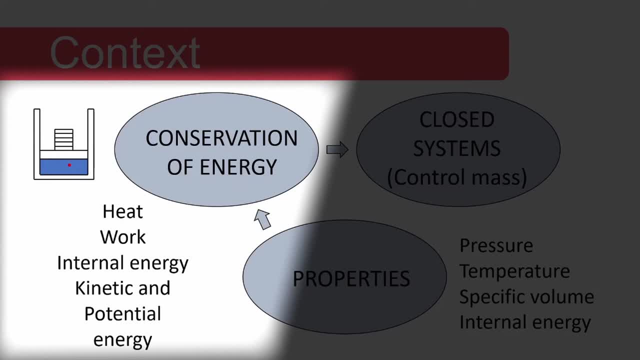 internal energy. Also, if the center of gravity of the control mass, shown here by the little red dot, moves during the process, we may also need to take kinetic and potential energy of the control mass into consideration. And lastly, we applied the first law to closed systems. 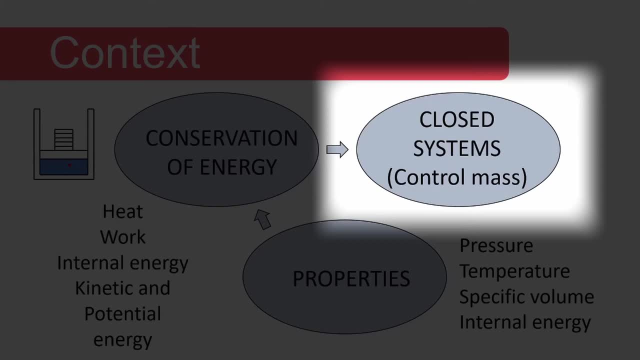 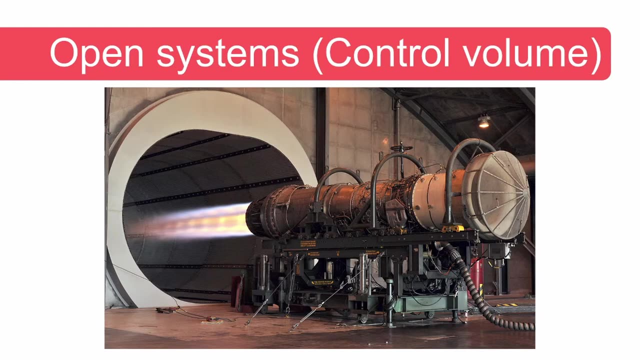 In a closed system, there are no mass transfer across the system boundary and therefore the name control mass. Now in this video, we will begin the discussion of open systems or control volumes. In an open system, mass transfer across the system boundary takes place, and here you can see a. 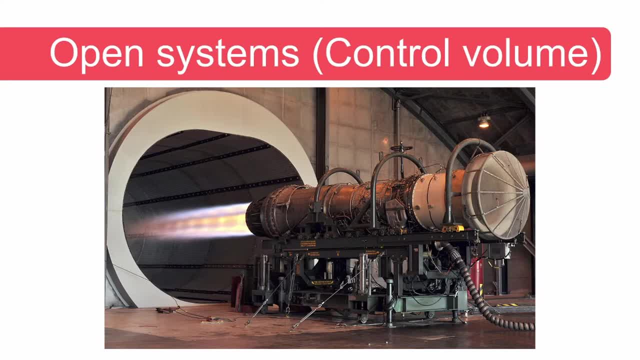 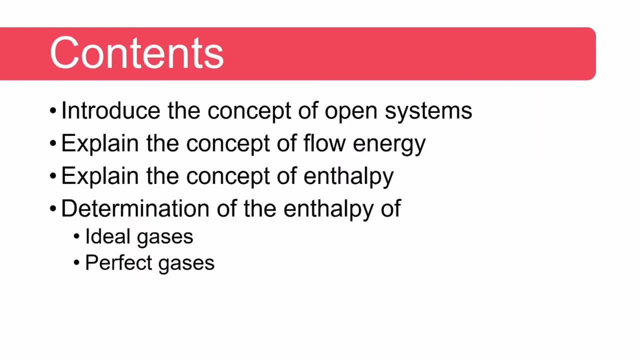 photograph of a jet engine on a test stand. Air and fuel flow into the jet engine and the combustion products flow out of the engine at high velocity. So the contents of this video then includes an introduction to the concept of open systems. We will explain. 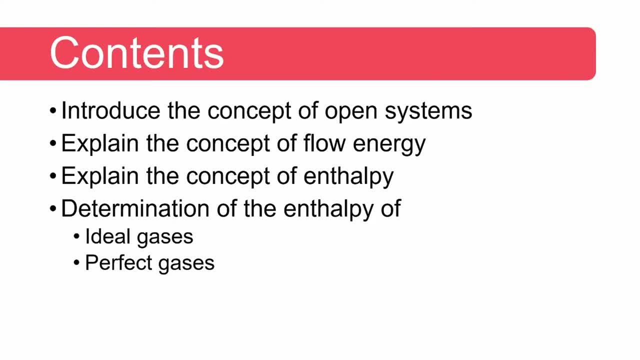 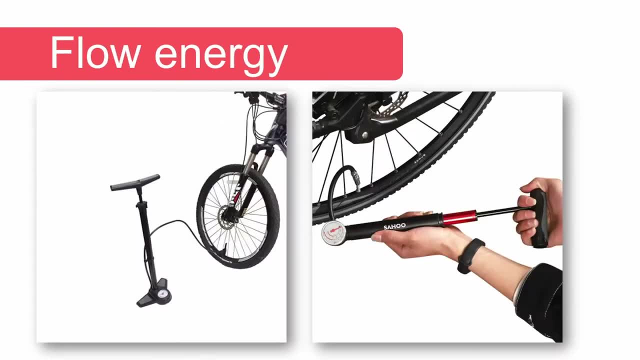 the concept of flow, energy and enthalpy, and then we will explain how to calculate the value of enthalpy for ideal and perfect gases. When we inflate the tire of a bicycle, we need to pressurize the air in the pump in order to force it to flow through the connecting tube into the tire. We 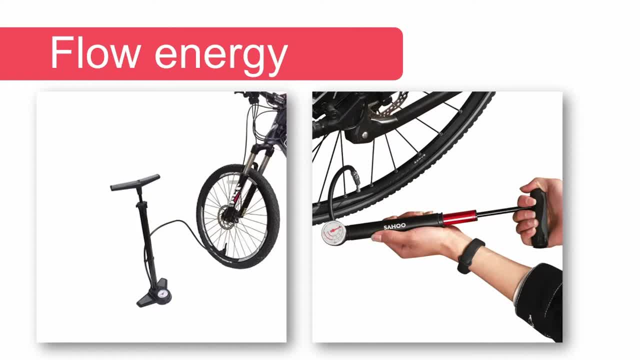 perform work when pressurizing the air. If we assume the pressure inside the pump stays constant, the work necessary to force the air into the tube is equal to the pressure inside the pump multiplied by the volume of air that flows into the tire. Work is a form of energy, and this energy 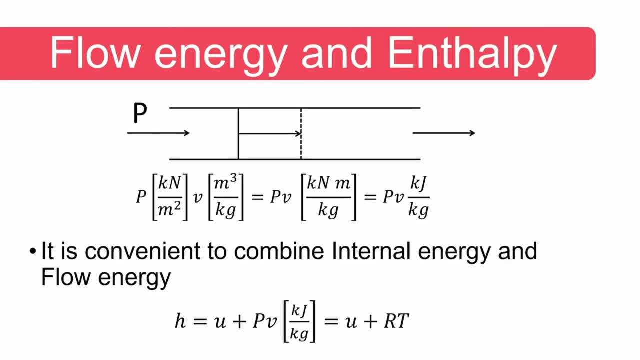 is called flow energy. Therefore, the energy required to cause one kilogram of fluid to flow is equal to p multiplied by the specific volume of the fluid and is called flow energy. It is convenient to combine these two types of energy, And internal energy and flow energy- into one variable, enthalpy. Enthalpy is an intensive 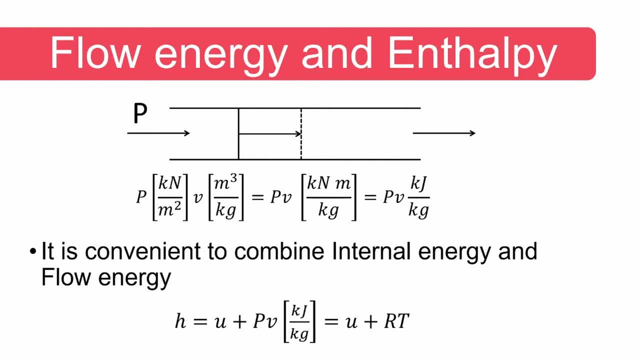 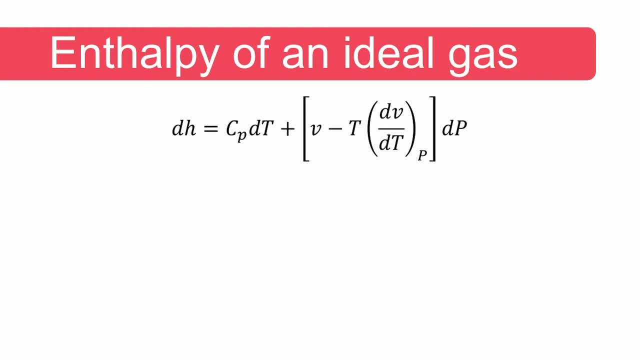 variable. Let us see how the enthalpy of an ideal gas is calculated. So the equation used to calculate enthalpy is given by the equation shown For an ideal gas. the term in square brackets reduces to zero and the enthalpy of an ideal gas is only dependent on temperature. Let 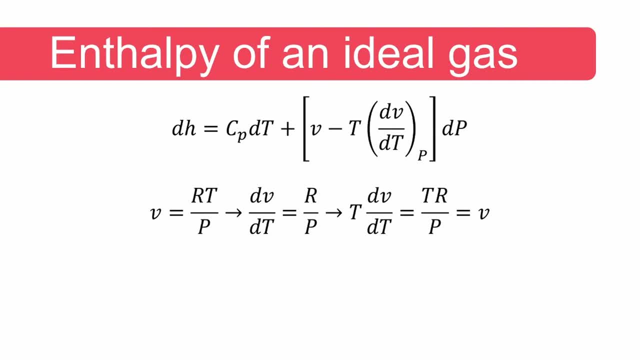 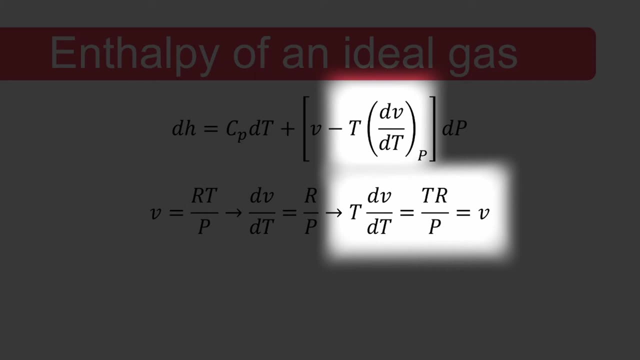 me show you why. For an ideal gas, specific volume equals rt divided by p. Therefore, the differential dv dt equals r divided by p, and t multiplied by dv dt equals tr divided by p, which is also equal to specific volume. And that's specific volume. 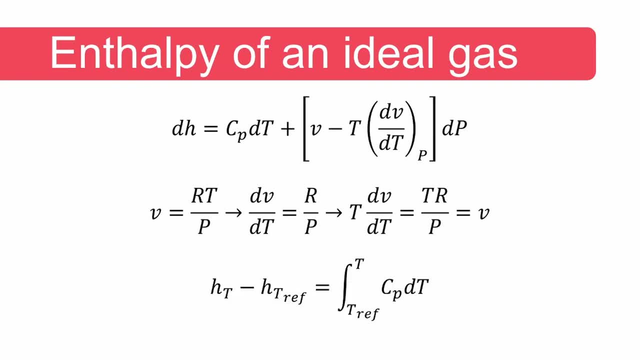 subtract specific volume equals zero. From this we then obtain an equation that enables us to calculate a value for enthalpy relative to a reference value, a reference temperature In general. the specific heat of an ideal gas is not a simple equation and the integration is not trivial. We do not want to perform the integration every time we need. 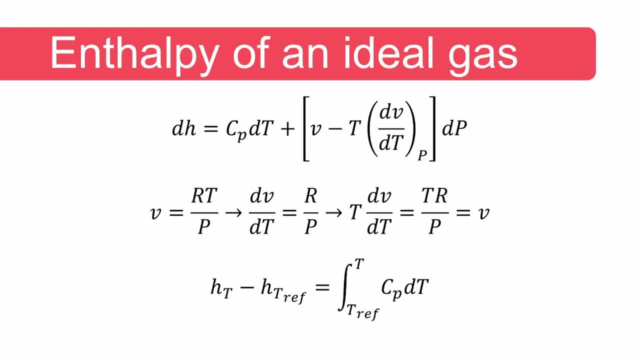 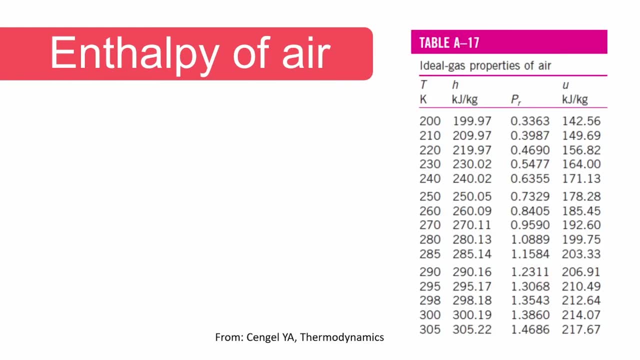 a value of enthalpy. So, therefore, the integration is performed for common gases under the assumption of ideal gas behavior and the values are tabulated. Now let's consider air. The value of enthalpy of ideal gas, such as air, as a function of temperature is found in the tables, As in the case of internal 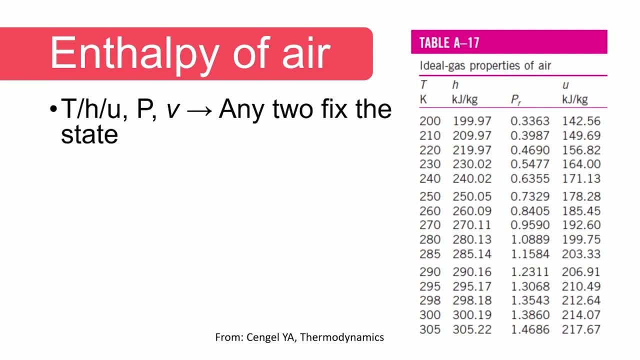 energy, the enthalpy of air is a property and if we know the value of two independent properties, we can calculate the value of the other unknown properties. It is important to note that in the case of an ideal gas, the values of temperature, internal energy and enthalpy are not independent. 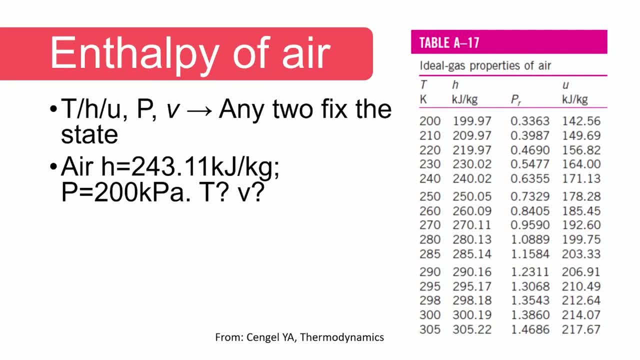 and the value of only one can be specified independently. Let us do an example. The enthalpy of air at 200 kPa is 241.1 kilojoules per second. The value of air at 200 kPa is 241.1 kilojoules per second. 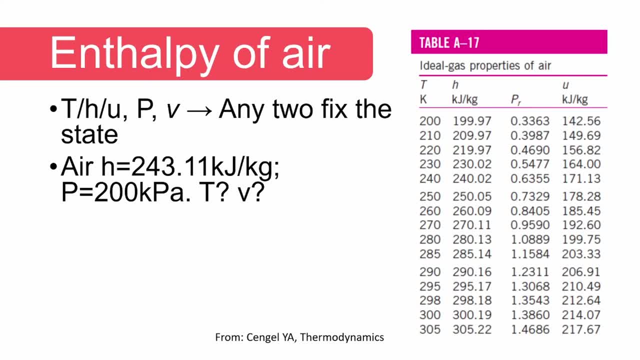 Now determine the values of temperature and specific volume. We can solve this problem by using the table. We see that the enthalpy values applied to us is between two of the tabulated values and we will have to interpolate to find the temperature of the air. See if you find the. 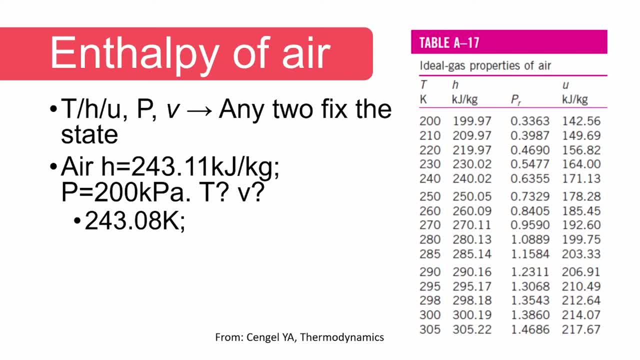 same value as me. We can then use the ideal gas law to determine the specific volume. Note that temperature, enthalpy and internal energy are not independent of each other. Once you specify the value of one, you can use the ideal gas law to determine the specific volume. Note that the 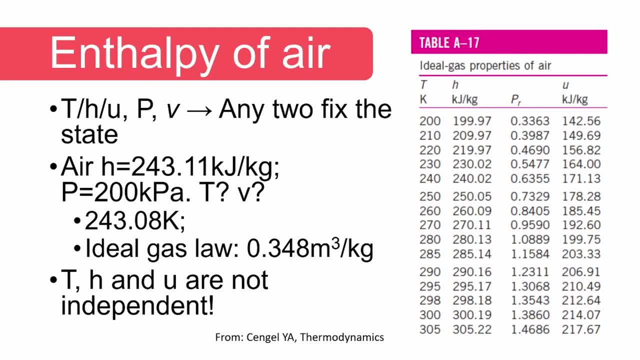 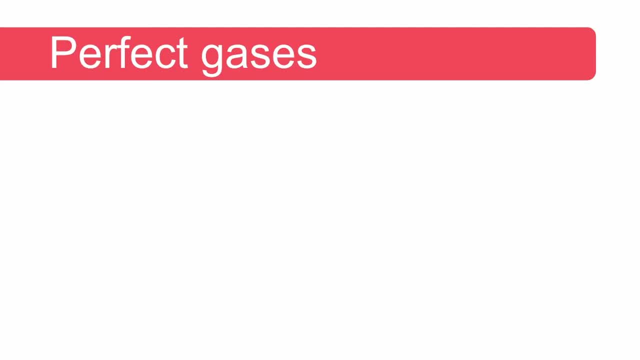 other values are fixed. Now let's consider a special ideal gas. If the specific heat of an ideal gas does not depend on temperature, we call such a gas a perfect gas. We often assume that helium and other monoatomic gases are perfect gases. For a perfect gas, it is easy to perform. 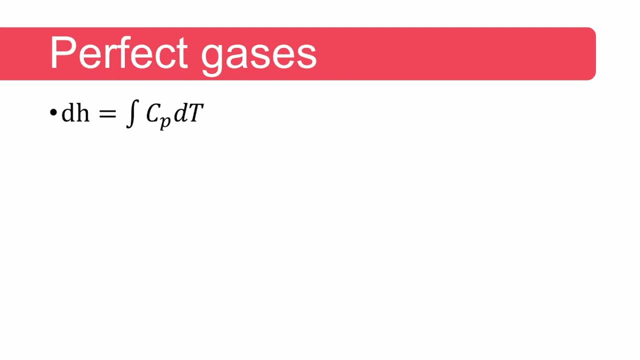 the integration of the equation for the calculation of enthalpy. The specific heat can be taken out from under the integral and the following equation results: Under the perfect gas assumption, it is important to know the temperature of the air at 200 kPa. The temperature of the air at: 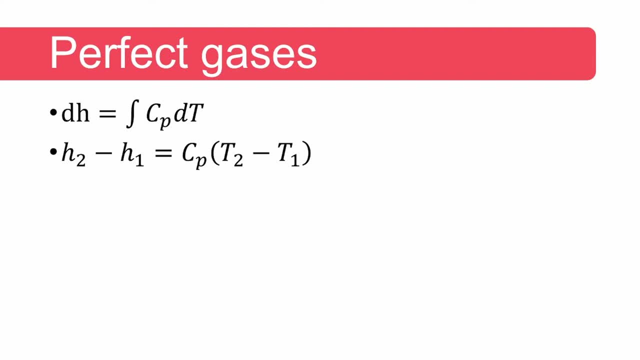 200 kPa is less than the energy of helium and other molecules. The temperature of the air is less than the energy of helium and other molecules. It is important to note that we now can only calculate the change in enthalpy. If we were asked to calculate the value of enthalpy for helium at 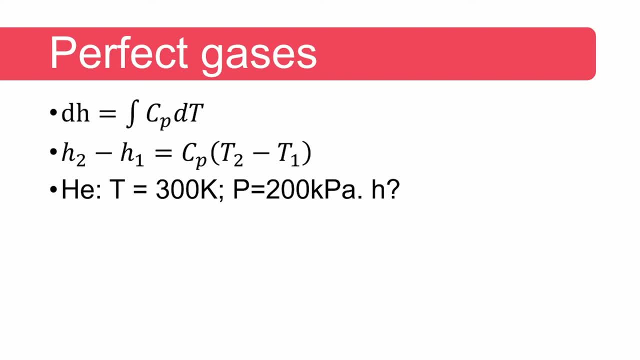 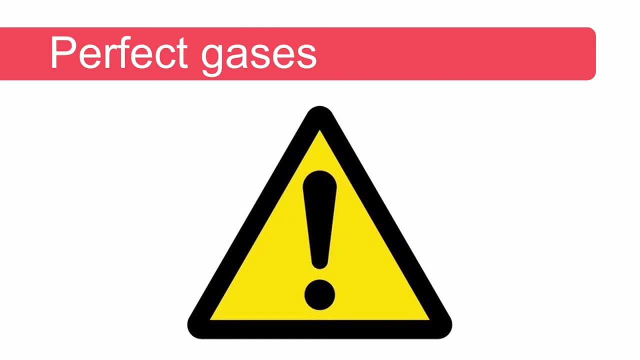 300 Kelvin and 200 kPa, we would not have been able to do it. Now you need to watch out. A common mistake is to assume perfect gas behaviour for steam and use the value of CP for steam found in tables to calculate the change and even enthalpy itself for steam. Now take note. 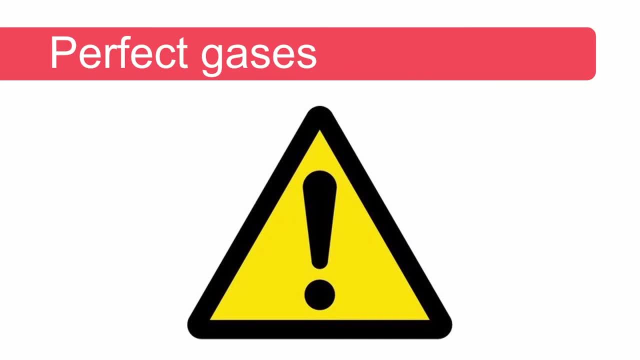 of the following. First, the value of CP in the tables is under the assumption of ideal gas behavior. only under very specific conditions, which is low pressure and high temperature, the assumption of ideal gas behavior is valid. secondly, in general water can undergo a phase change. an ideal gas does not change phase. the specific heat of liquid water differs to that. 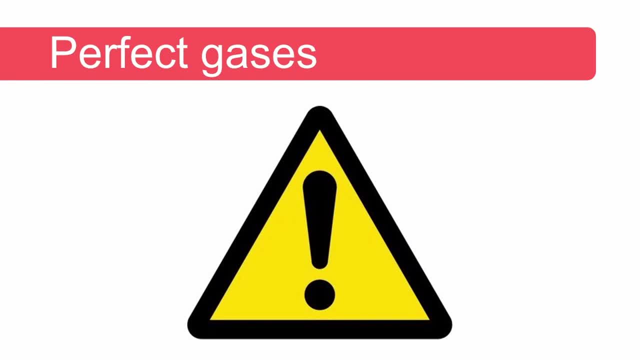 of steam, and cp does not take latent heat into consideration. thirdly, the tabulated value of cp is usually for a specific temperature. the specific heat for steam is not independent of temperature. so if you have not checked that the ideal gas assumption is valid under all circumstances for 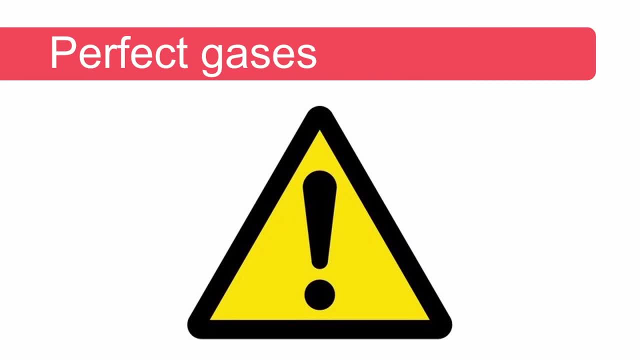 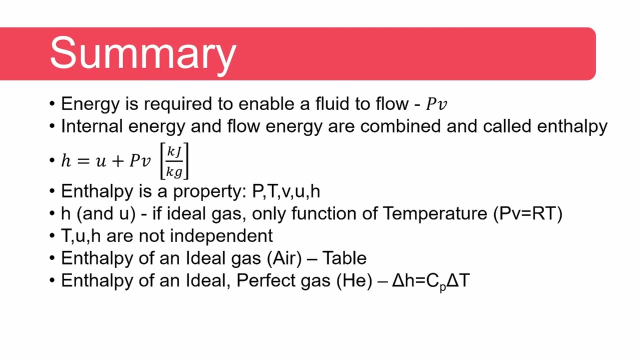 your situation and that the temperature does not vary too much. do not use cp to calculate the enthalpy of steam, and at no stage in this video playlist will we be assuming ideal gas behavior for steam. okay, to summarize: energy is necessary to enable a fluid flow. we can 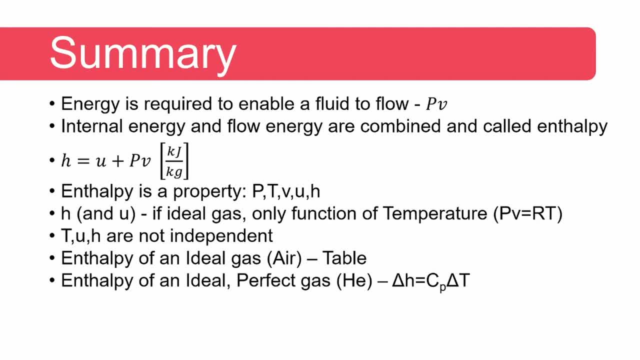 call this flow energy. pressure multiplied by specific volume, internal energy and flow energy are usually combined to form a property we will call enthalpy. enthalpy is a property and we now have five properties: pressure, temperature, specific volume, internal energy and enthalpy and in general.